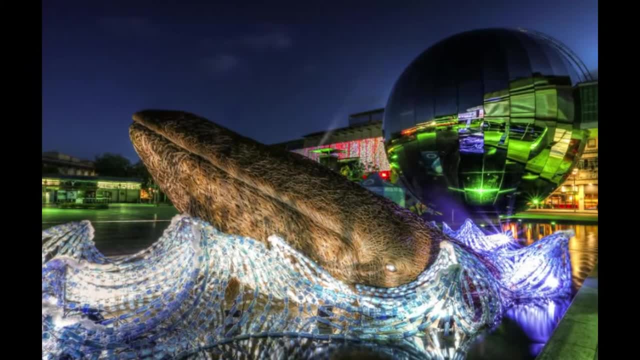 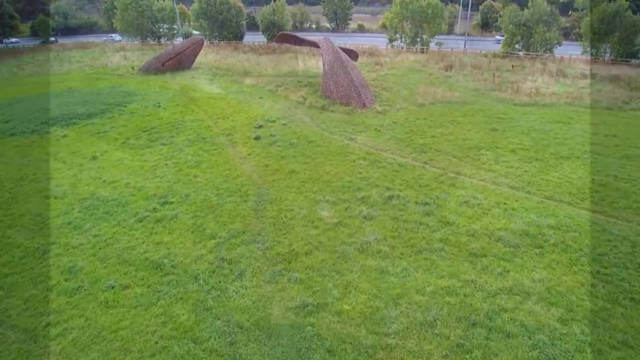 oceans. Upon its initial date, the art installation was created in 2015.. The art installation was created in 2015,, and the whale head seen above was surrounded by a sea of illuminated plastic bottles. The artwork was then moved to a nature reserve off a major highway, where it is slowly. 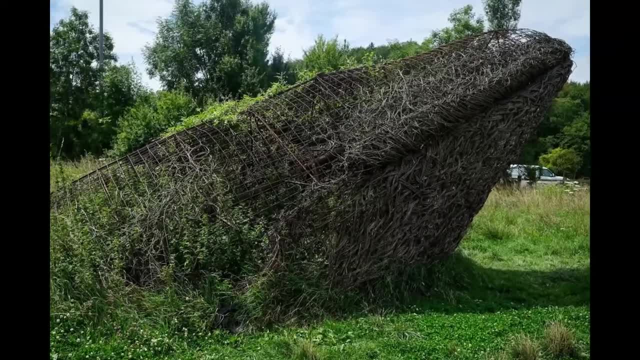 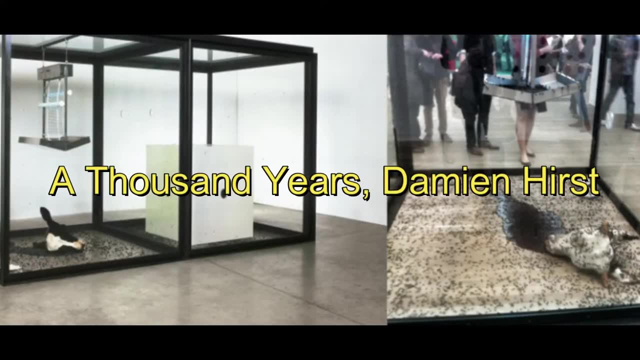 being taken over by nature. Who knows how much longer these whale sculptures will retain a likeness to their original state they had back in 2015.. Number 7, A Thousand Years by Damien Hirst. This is definitely the most macabre entry on this list. What the hell is that, you ask? Is that a? 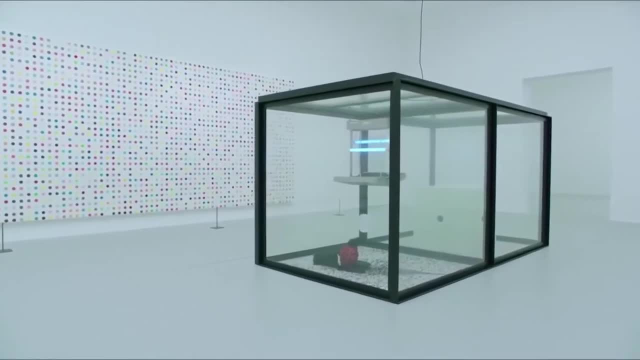 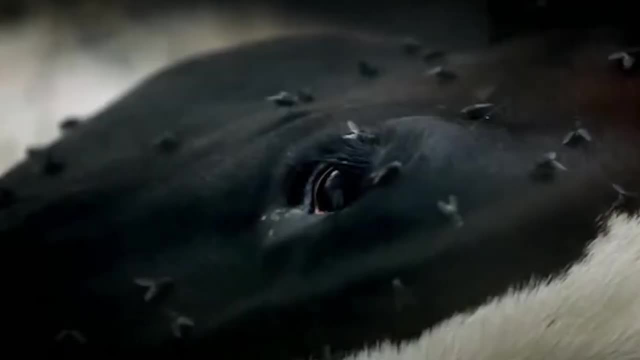 rotting cow head decomposing in a glass display surrounded by a sea of plastic bottles. This is glimpse of a bite-sized hanged bird having a heart defect and being bitten by hundreds of buzzing flies. Of course, Hirst created this temporary art piece to symbolically portray the cycle of life. 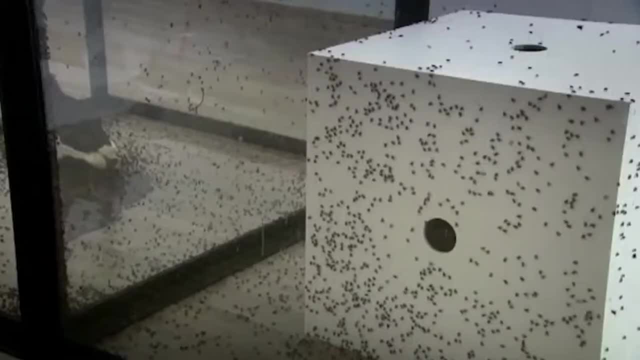 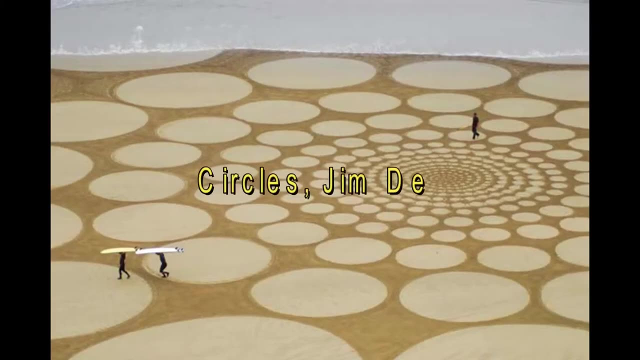 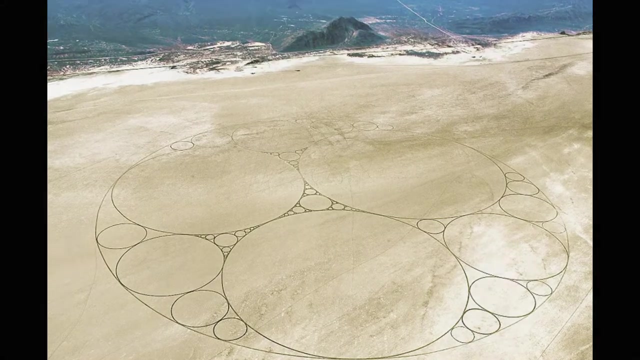 and death. The flies were also part of the life and death cycle, as they were eventually electrocuted and killed while they were on display in the glass vitrine Number 6, Sand Circles by Jim Denevan. This temporary sand art deserves a spot on the list for its massive scale alone. 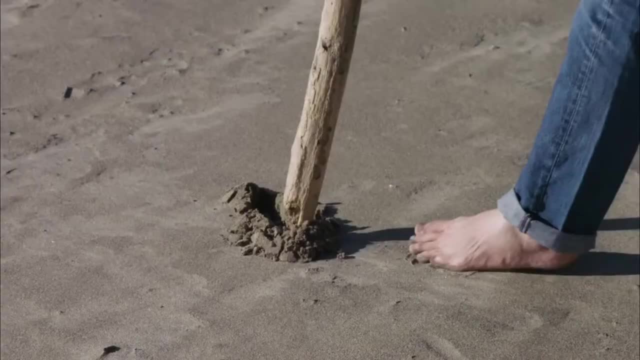 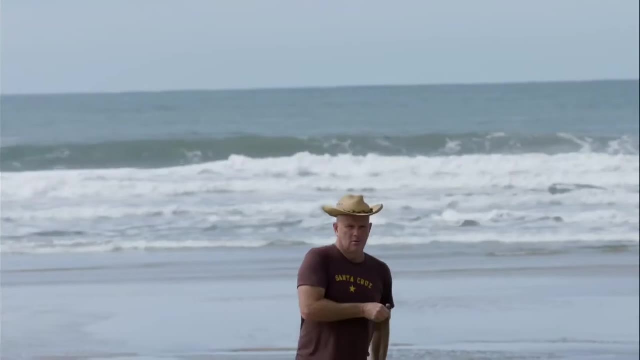 California amateur sand artist, Jim Denevan, created this impressive display of temporary sand, temporary artwork on a beach while the tide was out. As you can imagine, this artwork is only on display for a short time, as the tide will eventually come in and wash away all the 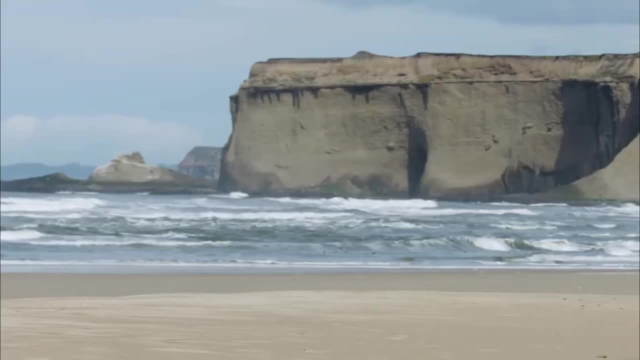 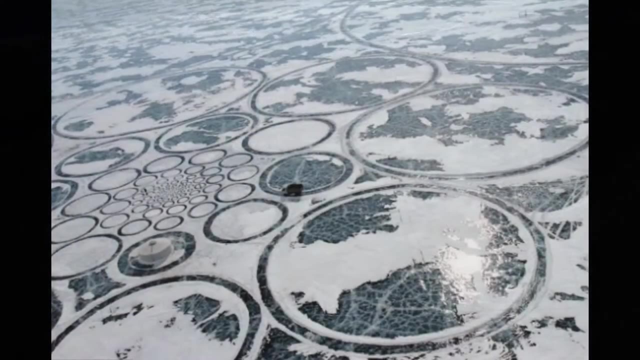 painstaking work that was put into it. Jim Denevan has created many pieces of temporary art over the years using only a stick, a rake, a beach and his imagination. He also created a notable piece of temporary art on Lake Baikal, which was designated as the world's largest single piece. 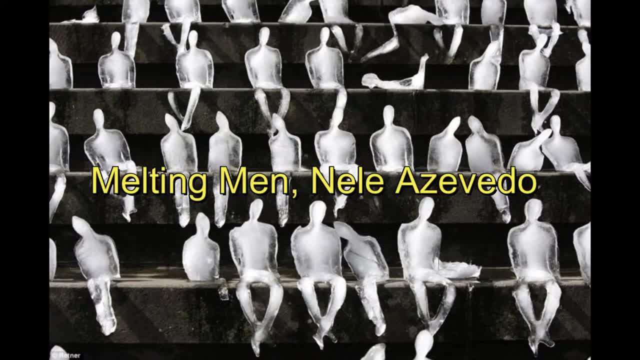 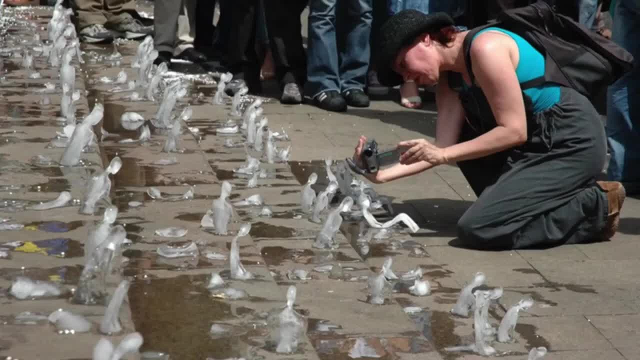 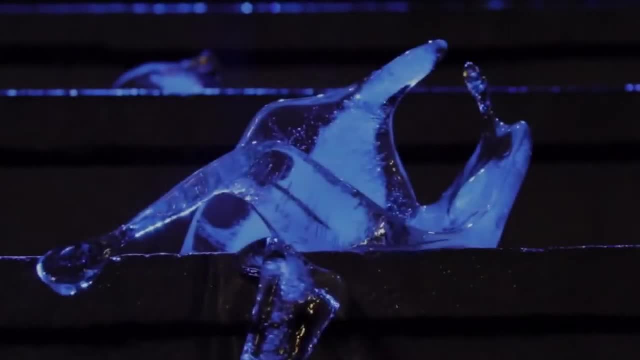 of artwork Number 5. Melting Man, Nele Azevedo. This art display was not just a singular sculpture, but consisted of 1,000 Icemen sculptures which slowly melted away before spectators in Central Gendarmenmarkt Square in Berlin, Germany. The temporary art sculptures began melting quickly. 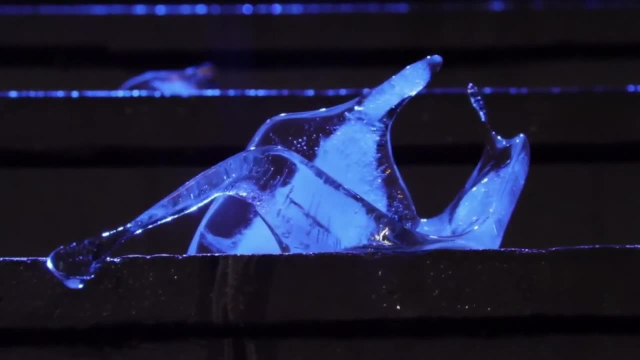 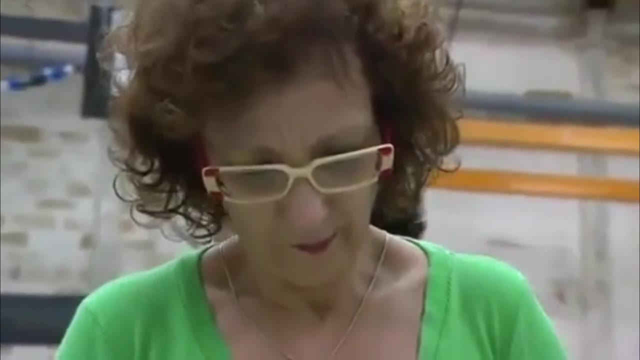 as temperatures reached 73 degrees Fahrenheit on the initial day of presentation to the public. The temporary art figures were crafted by Brazil-born artist, Nele Azevedo, to bring much needed awareness to the world of contemporary art. Nele Azevedo was the first artist to create. 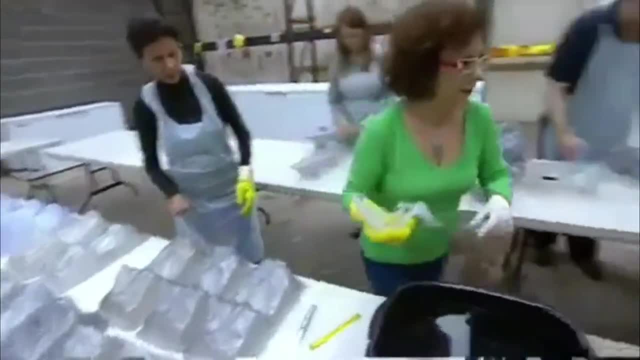 global art in the United States, and he was the first person to design a sculpture of his own. This was a great example of the power of temporary art and the consequences it can bring to mankind in the near future. Number 4. Key Biscayne, Sandcastle, Florida, This mind-blowing sand. 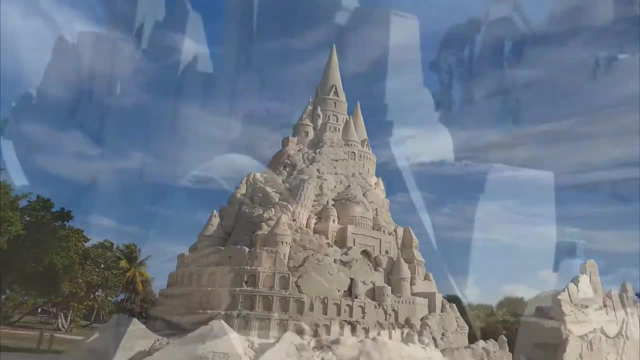 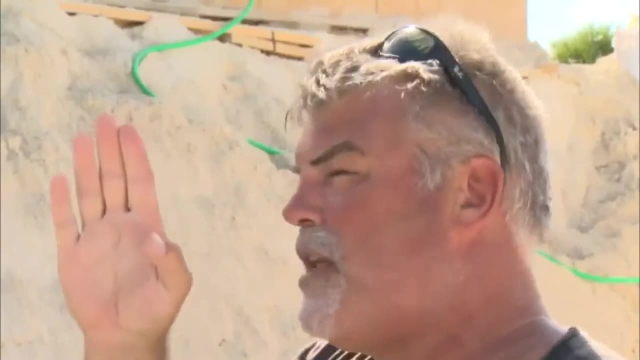 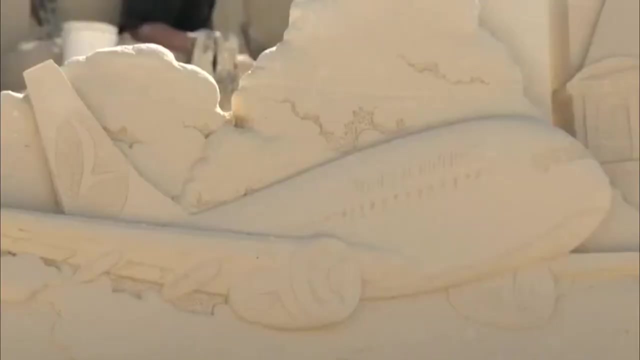 sculpture is the runner-up for the tallest sandcastle ever built. The temporary sand sculpture was constructed by a team of 19 artists in 2015,, led by world record holder and artist Ted Siebert. This sandcastle stood over 45 feet tall and consisted of 1,800 tons of sand. Back in 2015,, 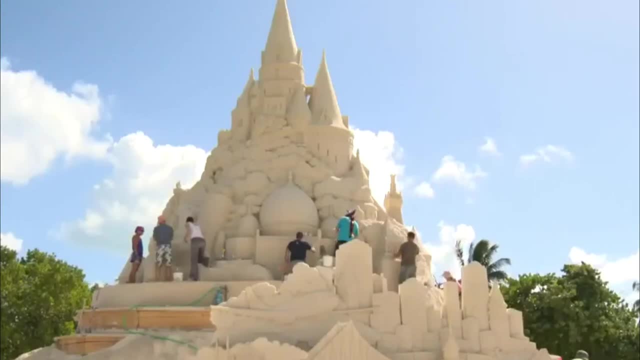 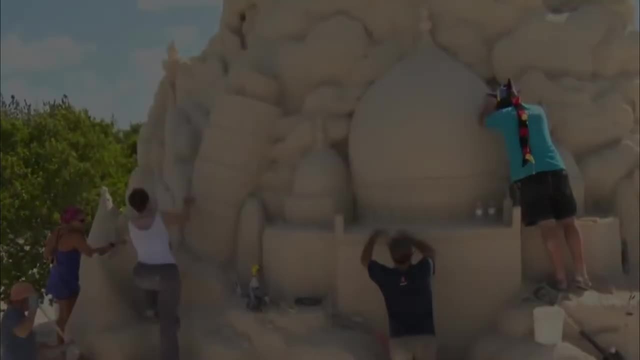 when it was constructed, it helped the city of San Fernando, California, and the city of San. it held the Guinness World Record for tallest sandcastle ever. This incredible temporary sand sculpture depicted many famous landmarks from around the world, including the Taj Mahal, the Leaning Tower of Pisa and the Statue of Liberty. 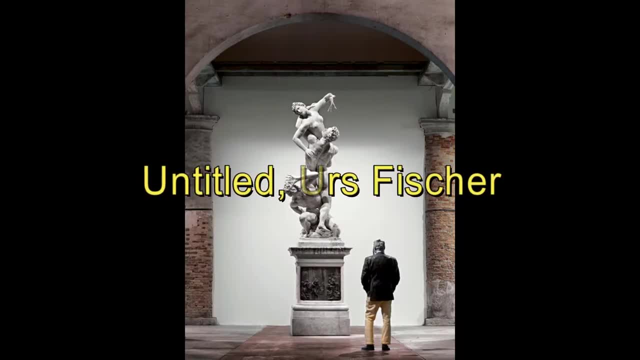 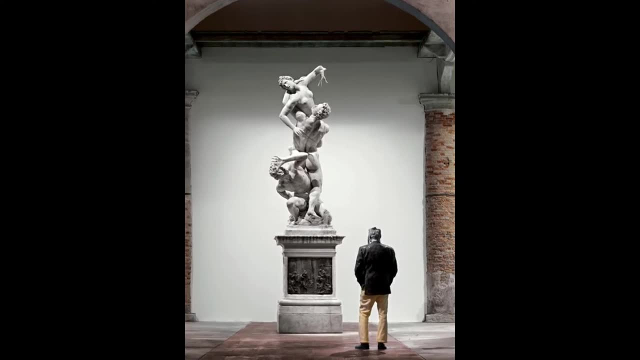 Number 3.. Untitled by Urs Fischer, Melting Candles. Don't let your eyes deceive you. This artwork is made of wax. Yes, even that man gazing upon his work of art in the lower right hand corner is part of the exhibit. 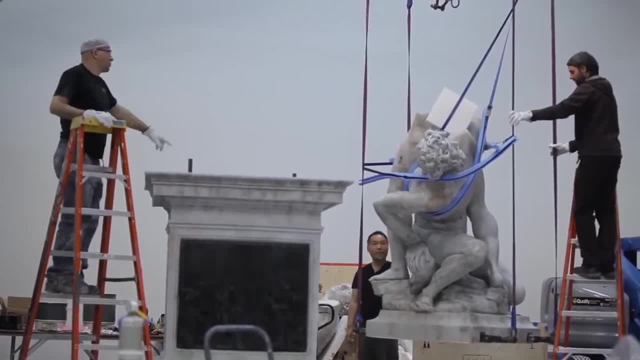 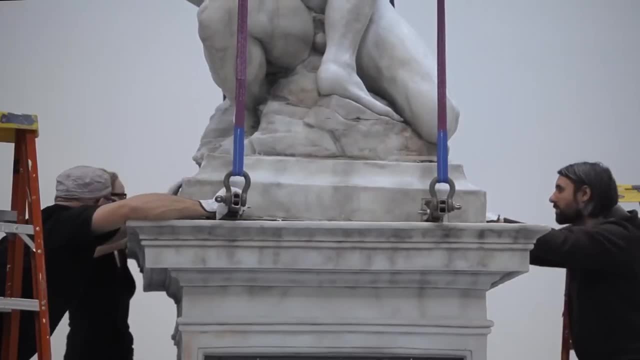 You can see his head beginning to melt if you look closely. This was a replica of a famous sculpture that was created for the Venice Biennale Art Exhibit back in 2011, and it was only on display for around five months. New York-based artist Urs Fischer poured his heart into this temporary yet intricate candle wax statue. 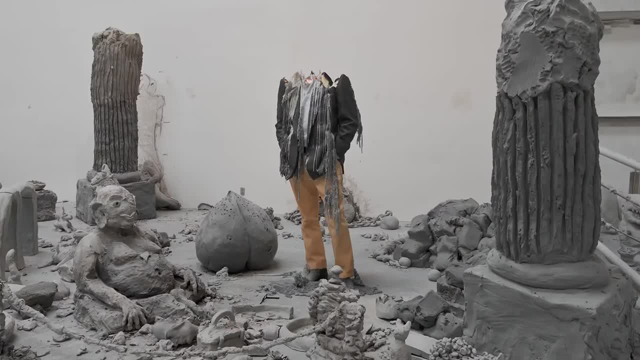 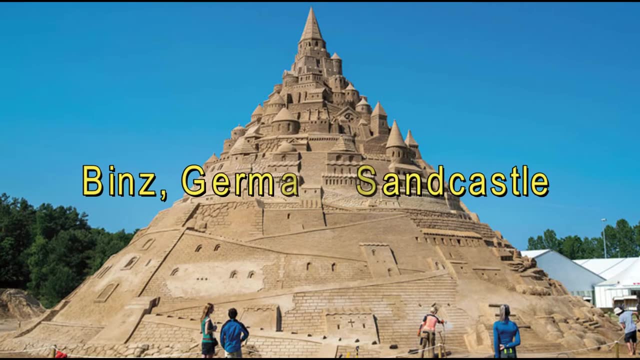 before it slowly melted away into a puddle of liquefied wax on the floor of the Venice Biennale Art, Exhibit Number 2.. Binz, Germany, Sandcastle- The world's tallest sandcastle. Seeing people standing at the base of this incredible sandcastle gives you some perspective. 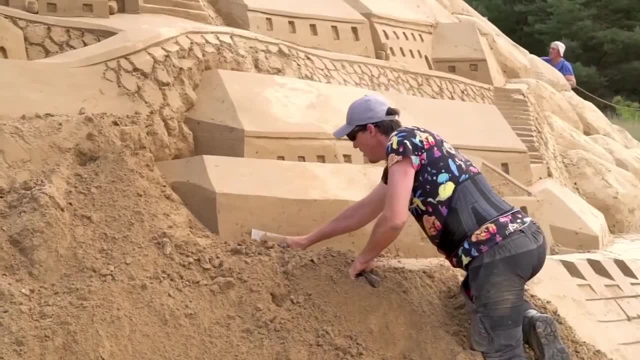 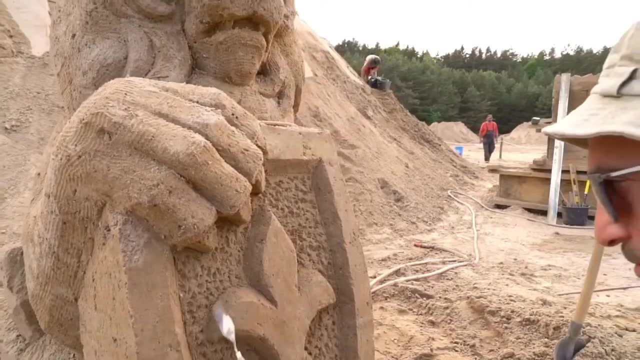 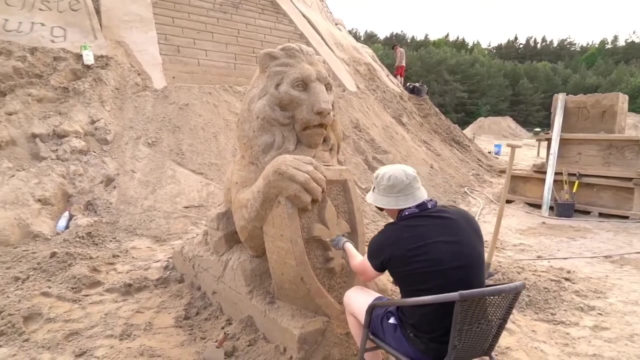 on just how massive it really is. Not only is it the tallest sandcastle ever created, this piece of art is extraordinarily detailed, right down to its last brick. This awe-inspiring piece of art was constructed by a team of international artists from all over the world for a sandcastle building competition in 2019.. 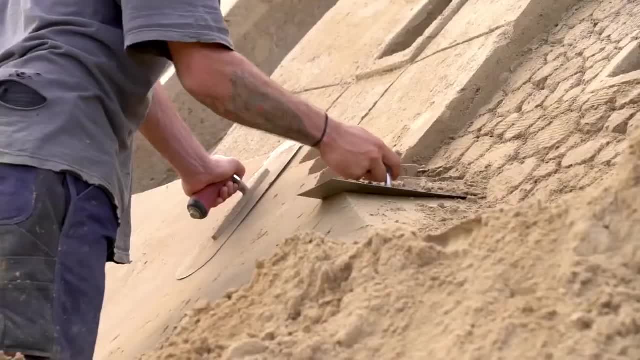 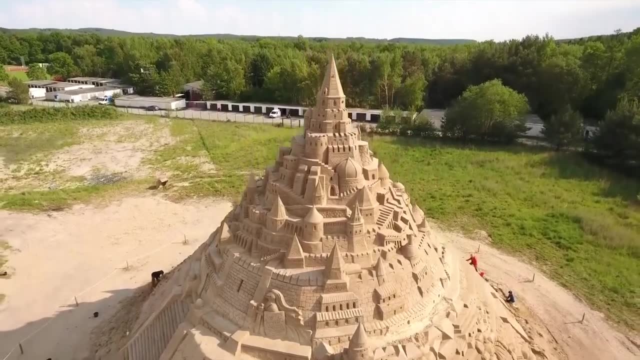 Unfortunately, the sandcastle only remained intact from May 2019 until November 2019.. The Binz sandcastle stood 57 feet tall and was recognized by Guinness Book of World Records as the tallest sandcastle ever built. The castle also came equipped with a large dragon carved into its base. 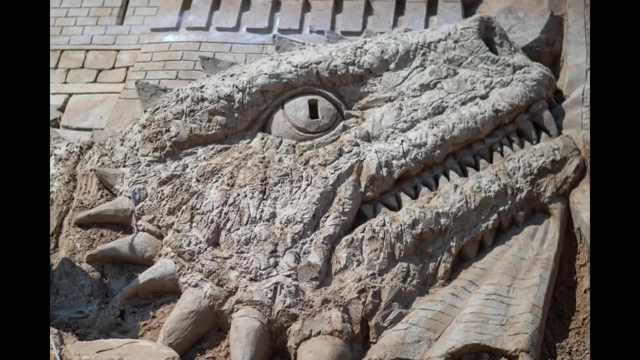 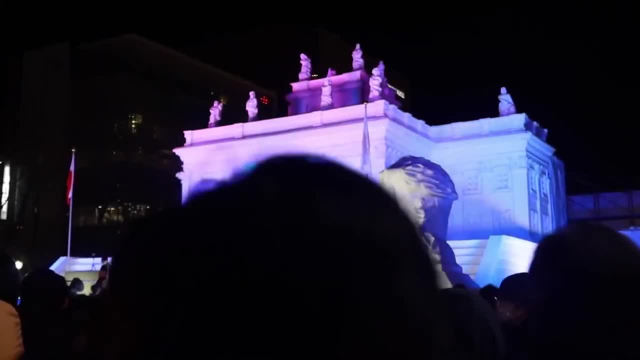 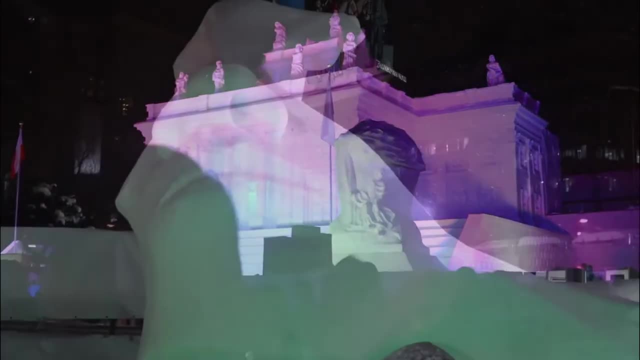 to go along with the Game of Thrones-inspired theme of the sculpture Number 1.. Palace on the Isle Ice Sculpture, Sapporo, Japan. This incredible ice sculpture was prominently featured in Japan's Sapporo Snow Festival, an annual festival that's held in a frigid northern Japanese city that is quickly becoming.